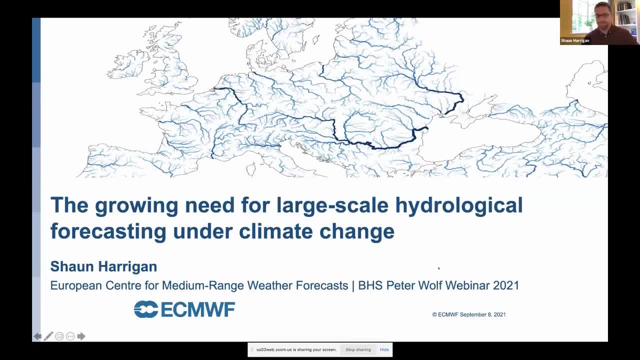 Thank you very much, Chris, and welcome everybody. So I'm Sean Harrigan from the European Centre for Medium-Range Weather Forecasts, based in Reading in the UK. I'm going to talk today on the growing need for large-scale hydrological forecasting under climate change. 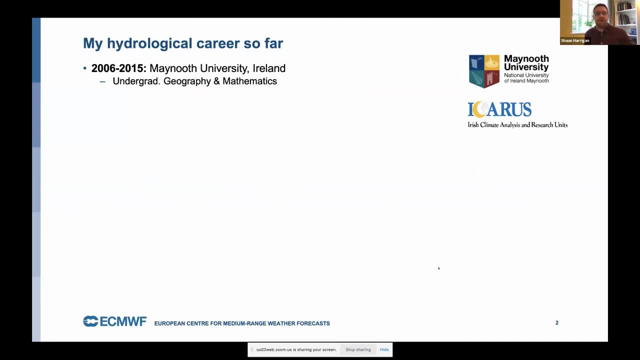 So just a little bit about myself first and my hydrological career so far. So, as you can tell from the accent, I'm originally from Ireland and that's where I did the majority of my studies, and through undergrad to PhD, and so really I think the story is: you know how did? 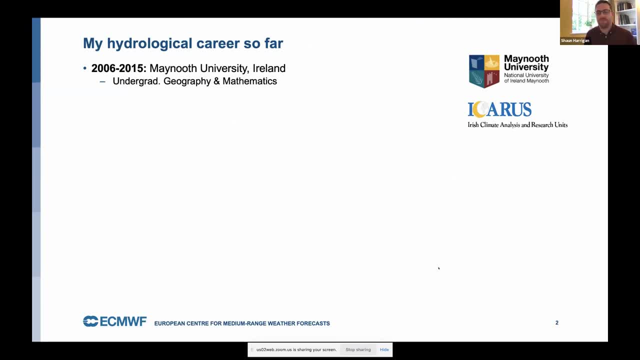 I get into a career in hydrology, and it wasn't obvious, by no means. it wasn't something I woke up one day and thought, as a young person, this is for me. I just stumbled across it based on my interest. I studied geography and maths at university and just naturally, 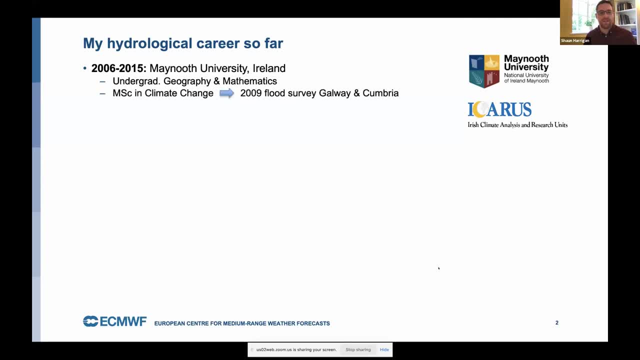 liked numbers and liked how the world works, and so that kind of piqued my interest in both climate and hydrology- the two joint subjects That led me on to a master's in climate change that I was able to study hydrological components in, which was what I really wanted I'm going to go through. 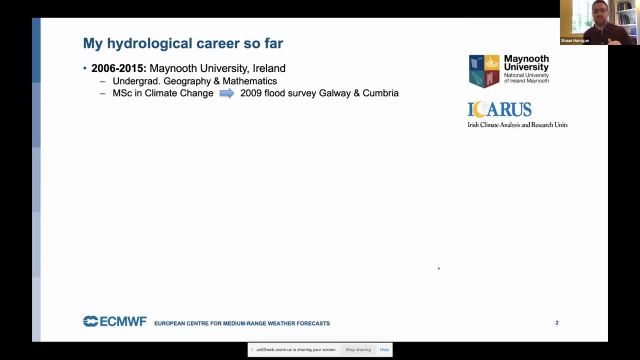 a couple of kind of lessons or kind of key things along my journey, kind of as a hydrologist, that I think were quite important for those who are maybe on that, on that path as well. So, even though I was studying a lot of the science, I got the opportunity to be involved in a flood survey based on the 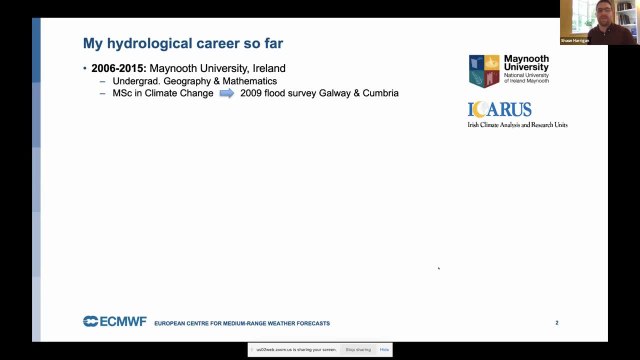 November 2009 events. Flood event that affected both the west of Ireland and the northwest of the UK and Cumbria, and that survey was actually more almost a social science experiment than a scientific one, but what it really taught me was the importance of the event and the kind of 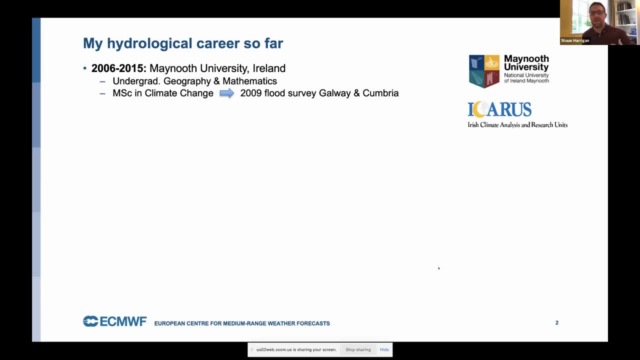 human impact these floods have on people and that really helped me kind of. it kind of really brought what we're studying and the numbers we're running and the models we're running and observations we're analysing into the fore and the importance of the work we're doing and 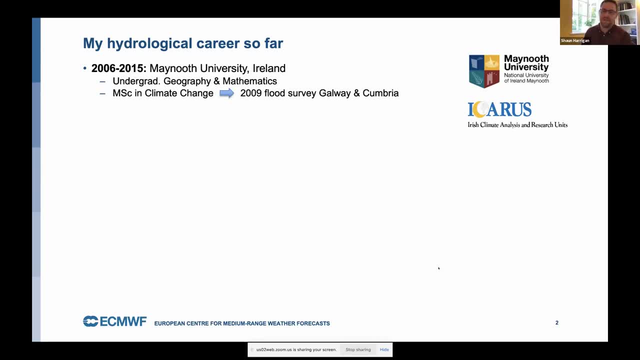 I think that was quite important and kind of deciding where I went next. I wasn't quite sure after my master's whether a PhD was for me. I liked the research element but I just wasn't sure was a PhD the right option? so instead I spent, took a year out and 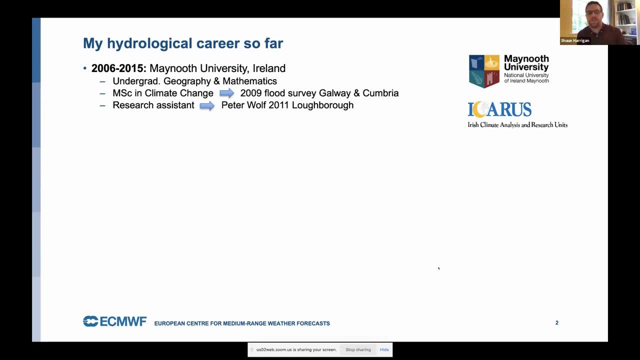 worked as a research assistant within one of the research centres at the university, at Chris Irish climate analysis and research units, and so there I got a chance to actually work on a research project being paid, and that's the first time I actually came across to the Peter. 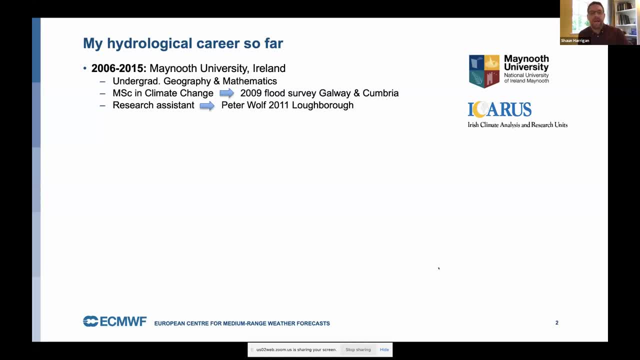 Wolfe event, so that's over 10 years ago now. it was in Loughborough and working with Rob Willoughby and colleagues. there was a, you know, a really important part actually of my development and in terms of then moving on to a PhD and working with my supervisors- and Rob was also working on that project. 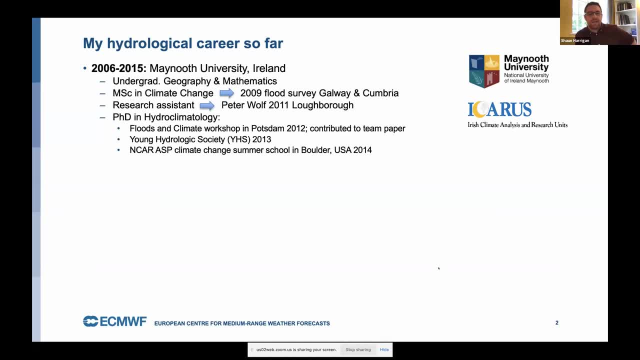 and so that brought me on to a PhD in hydroclimatology, and so that's when I kind of brought my two kind of interests in climate and hydrology together and and just three things I'm looking back at my PhD- that I felt were really important. and you know we're talking about innovation today and sometimes innovation can of 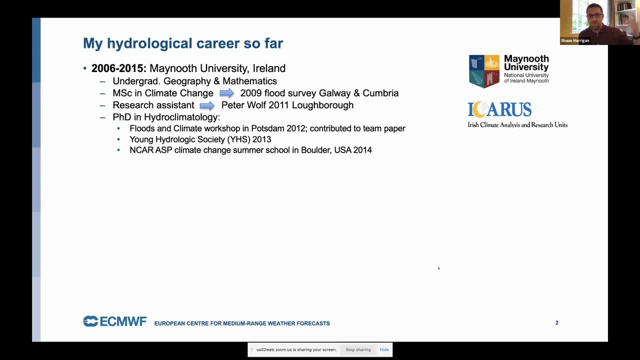 course, be ideas and be like a scientific thing that I was working on, but often PhDs you're. very few people have the opportunity to be groundbreaking in terms of the work they're doing. often you're feeding away at a problem and you're making your individual contribution to that as best you can. 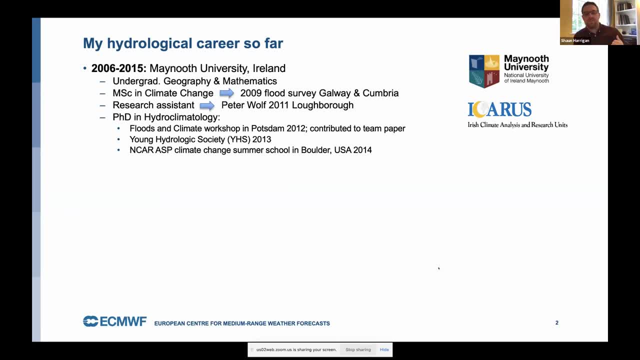 and so sometimes for me then, in terms of career, it wasn't this grand idea that necessarily that was, looking back, the most important thing- I think there were three main things that occurred- was one when it was very early on, just starting my PhD, and there was a 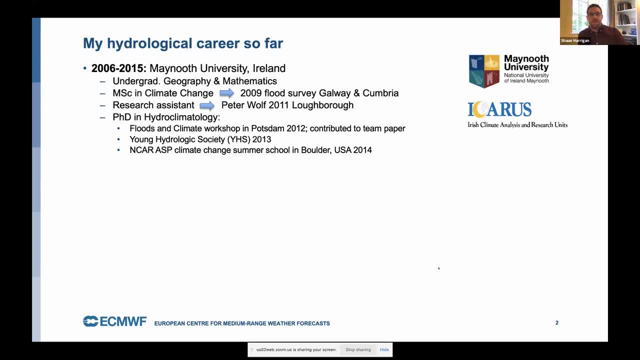 workshop on flows and climate in Potsdam in Germany and I remember going and it was a fantastic workshop- I decided that there would be a paper written, a clever paper- on a perspective piece And as a new PhD student, I you know the email came for contributions. 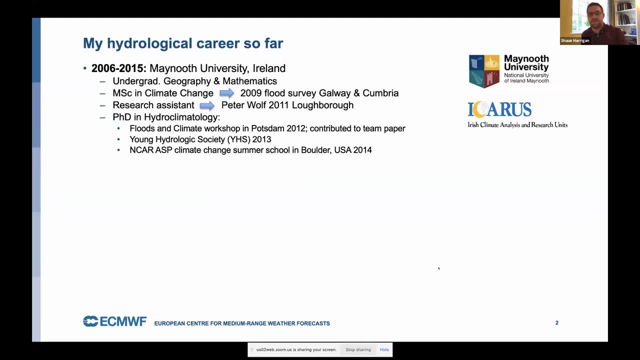 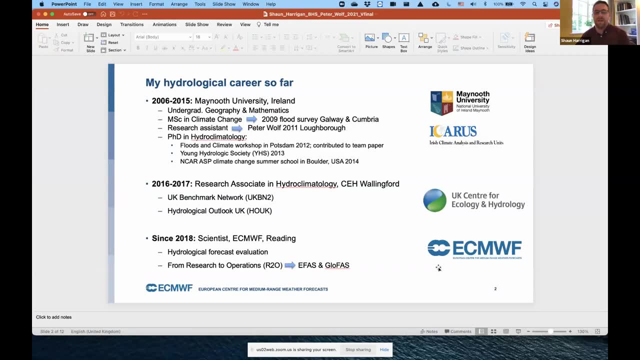 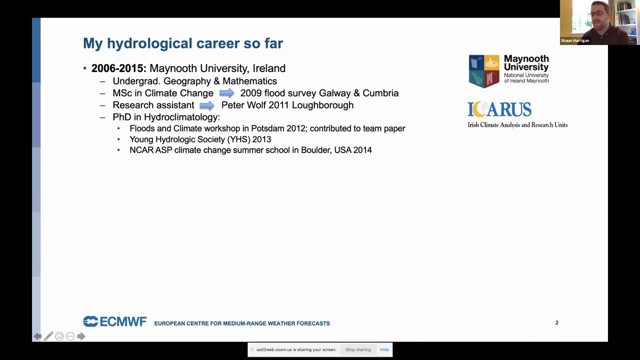 And I originally thought I have nothing to say, given this list of very famous authors. But I decided, I went back and just decided maybe I'll just chance write a paragraph and see what happens. And it turns out that that paragraph was accepted in the paper. 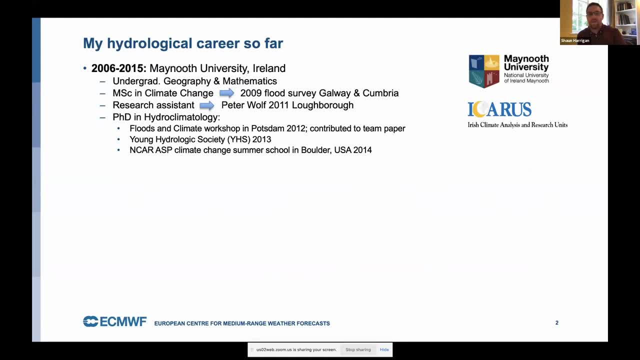 And that was. you know, I contributed an author and it's done really well And I think that was quite important to understand that you can make a small contribution to these large papers. You're valued to be said. The second thing: when going to look to go to conferences: 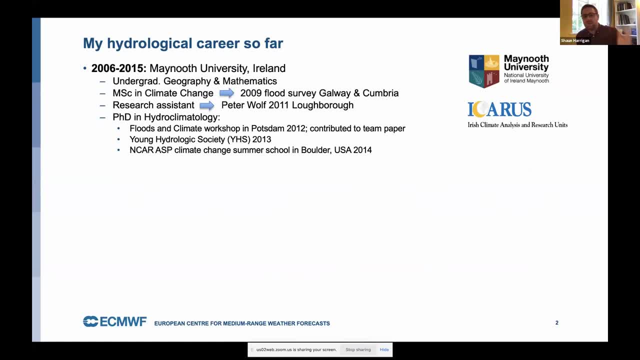 I didn't really know any people in the area working in hydrology. I was going to the EGU at the time, And so I seen a couple people wanting to start a new hydrological society for young people- early career scientists- back in 2013.. 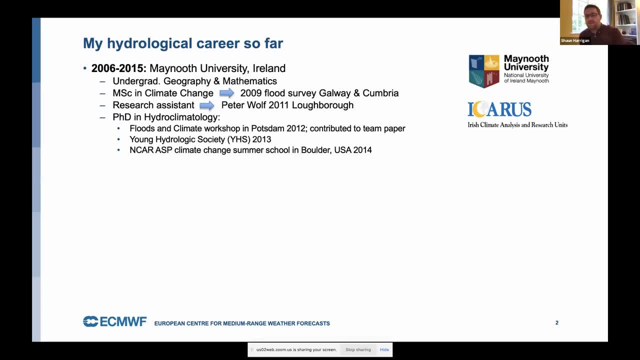 And I joined, just sent an email and got involved And that turned into be very, very important for building other colleagues and you know people that have collaborated with since, And that was the birth of the Young Hydrologic Society, which has, you know, is now compared to when, even back in 2013,. 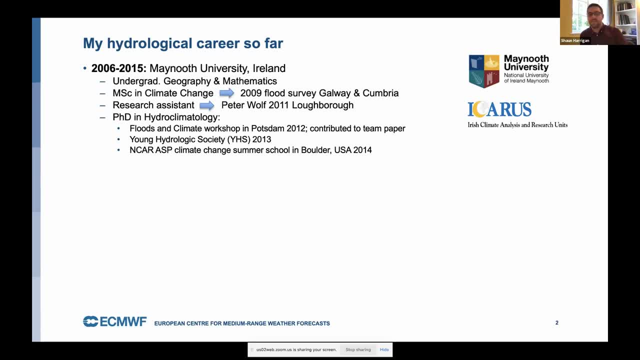 there wasn't very many early career events at these large international conferences, But if you go to one today- which we hope to do in person soon- you know that's quite common to have short courses and have dedicated events for early career scientists. 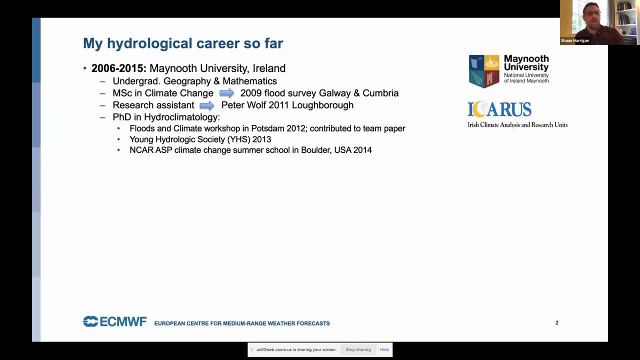 So I think that was a really important thing, just to get involved. If you see these initiatives, I think it's really valuable to just lend a hand and contribute. And then the third thing was I went to summer school at NCAR-ASP Advanced Summer Study Programme. 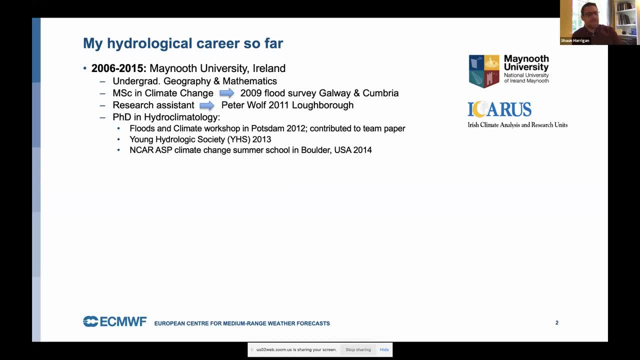 and climate change in Boulder in the USA And that was, from a scientific point of view, as well as collaboration with other scientists, really valuable, And so I highly recommend, if you see these opportunities, to just to apply. And you know, it's if you, if you are lucky enough to get selected, they're fantastic. 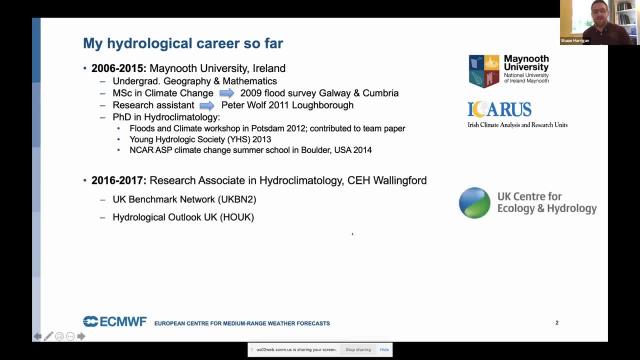 So that led me on to, you know, finishing studying and I had to decide whether to go into academia or go into research. I wasn't sure an opportunity came up to join a position, So I decided to go into research at the UKCH in Wallingford, the UK, as a research associate in hydroclimatology. 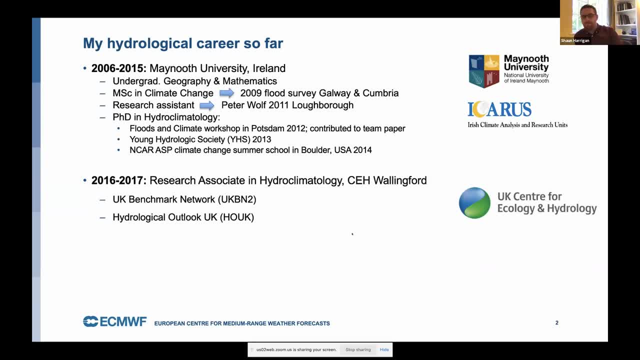 And there I worked on the UK Benchmark Network, which is a network of catchments for use for analysis of long term trends in the UK. But I think really important on what this led me into the area of hydrological forecasting through the Hydrological Outlook project. 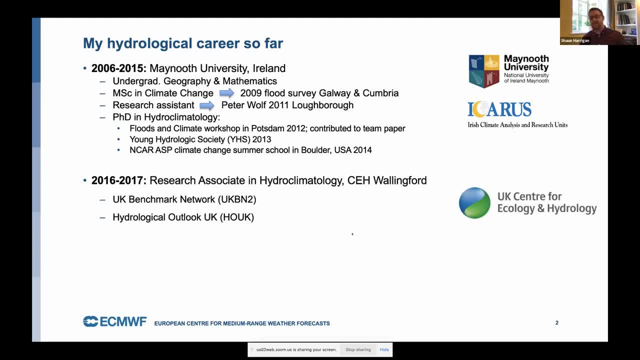 And so that kind of really piqued my interest And scientifically and just in terms of real world application. And that's kind of brought me to where I am now working at the European Centre for Medium Range Weather Forecasts, And so my role is working on hydrological forecast evaluation and what our key role is is bringing research to operations at large scale hydrological forecasting systems. 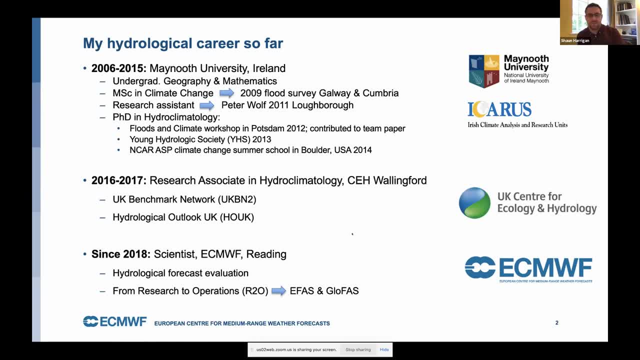 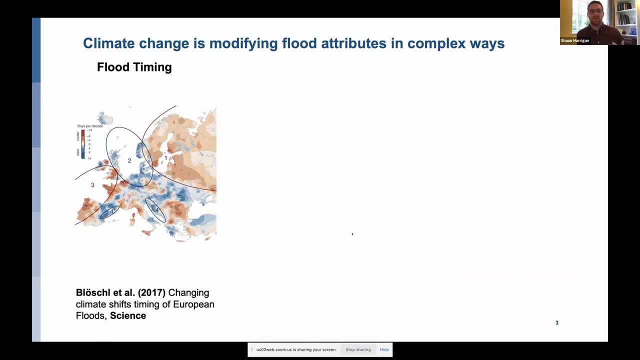 So the EFAS and GOFAS, which is the European Global Flood Awareness System- I'll speak a little bit about that next. And so just in terms of climate change and what, how that is modifying flood attributes, I think it's modifying in very complex ways. 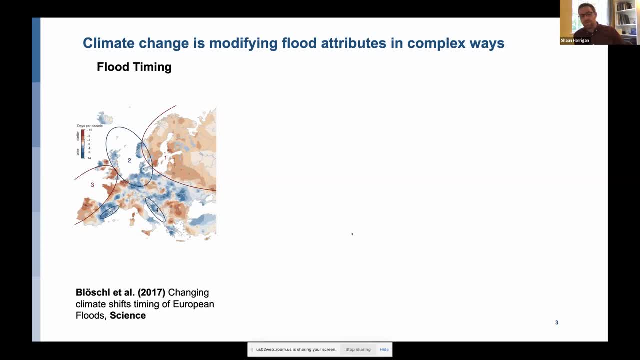 And so really, some of the early studies or the new studies that bring in these European networks of observations, have been able to show that we see changes in timing of flood events across Europe. That has either happened later or earlier than usual. We also see that the magnitude of floods are also changing, increasing in some parts of Europe, decreasing in others, so not necessarily. 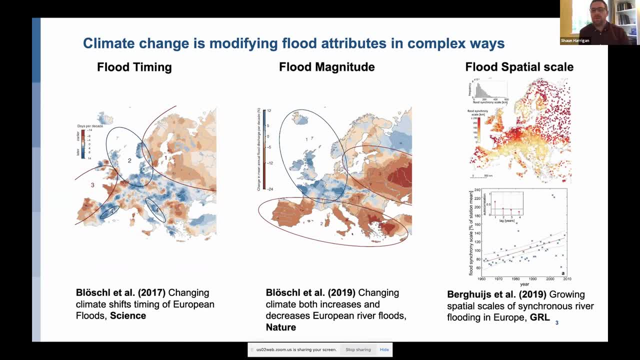 the same signal And other aspects of flooding. that I think is important, and why these large scale systems, in my opinion, are so important, is flooding does not occur in isolated events. It's not a single, often a single catchment floods. The most damaging events are multi-catchment, multi-country events. 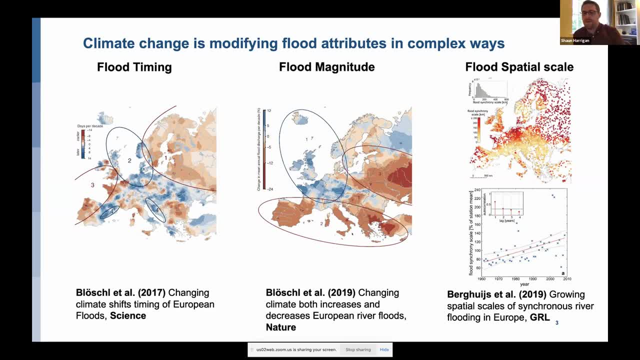 And we can see from this work that we've done with Vajabairkaus that if we look at this- the flood synchronicity, so when floods occur at the same time we can actually see patterns and mirrors across the continent- And when we look at the 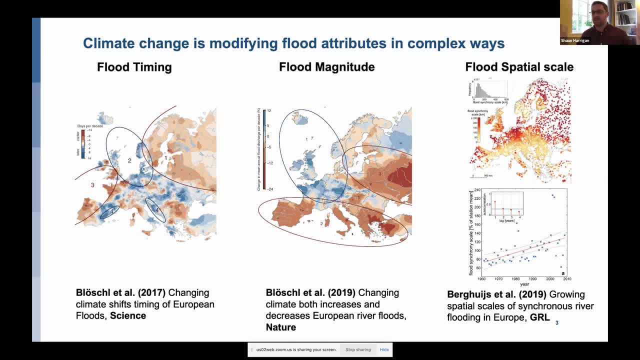 observations, we can see that the actual spatial extent of flooding is actually growing over time from the observations. so all these kind of changes, when we detect from observations, is implying that we are seeing changes. we need to understand them and we also need to manage them in terms of how floods are affecting society, and it's not easy. if we look at, then, the projections, 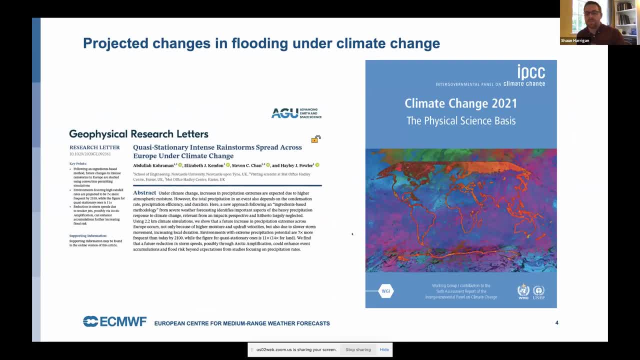 so what are we going to expect to see under a warming climate? and we see a fame? quite a well cited study and this summer was looking at stationary storms and these large-scale systems- that was, that were in some ways responsible for the the july uh flood that affected many countries. 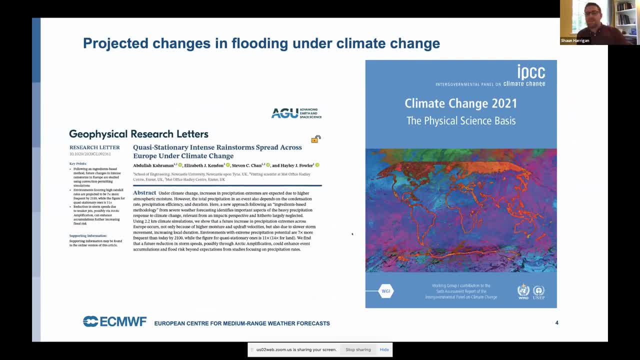 in europe, uh, this summer, and we see that some of these storms can be slow moving and attend within a warming climate can become stationary and stagnant, and this is very damaging. so the the news on that front, in terms of the atmospheric drivers, um, this is one example- is is not good news. 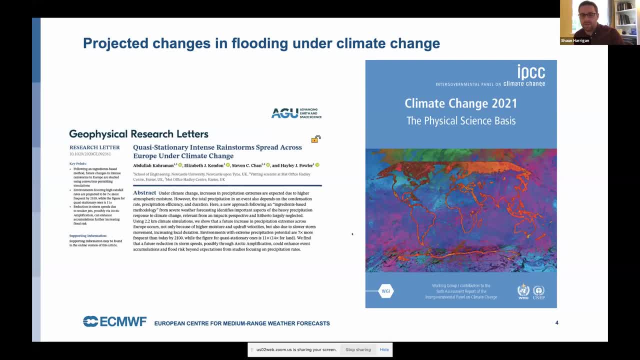 and we also, i would highly recommend, you know, having a look at the the new sixth assessment report from the ipcc, and chapter eight looks at the water cycle changes and indeed it's not very clear. there's no one obvious signal in terms of how floods are going to manifest under warming. 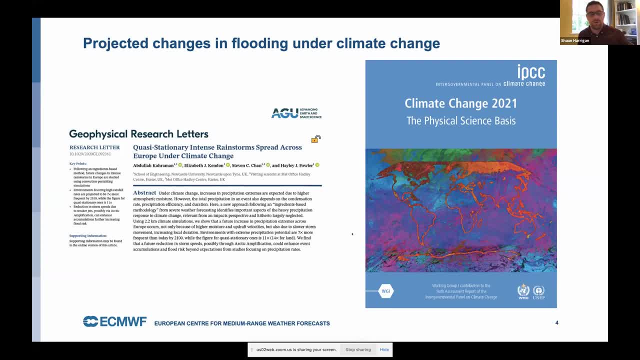 climate. it's complex with land and atmospheric and human kind of contributions, but the basics are there. you know the the water cycle is intensifying and when we these events occur, what we've seen from recent examples is entirely consistent with what we expect to happen. and this kind of brings us to to this event. 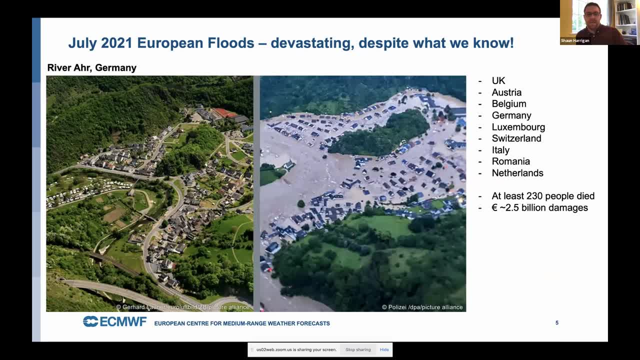 in terms of what's just happened. um, i'm sure you've all heard about this in the news. it was everywhere. um, it was devastating, despite what we know. i think that has the. the key thing that summarized it for me is: all the models we understand, all the data we have, all the signs we've been 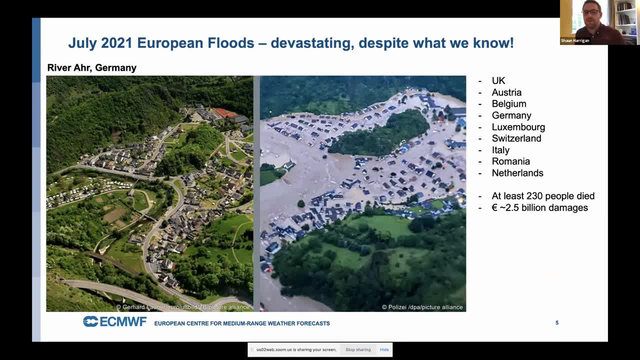 doing all the forecasting systems we've been put in place over the last 40 years, yet that there were still, you know, at least 230 people um died, at least 2.5 billion in damages and affected. you know. here's just a few countries that over that month were hit with the flood, not necessarily from the exact 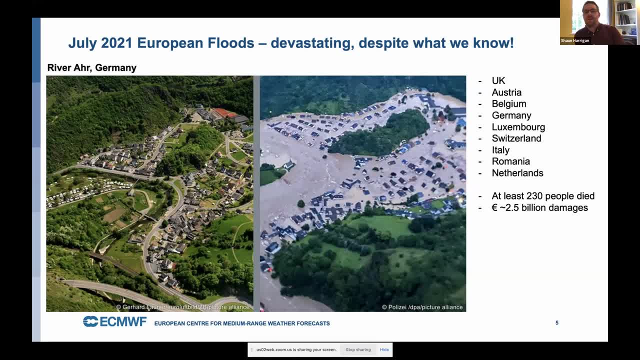 same event, but it was. it's complicated, but over that month we have, you know, nine countries here, you know, with severe damages ranging, uh, depending on which country, and, um, i i think for me that that, in terms of the, the kind of the shock of that system, it was a july event. okay, it was in the. 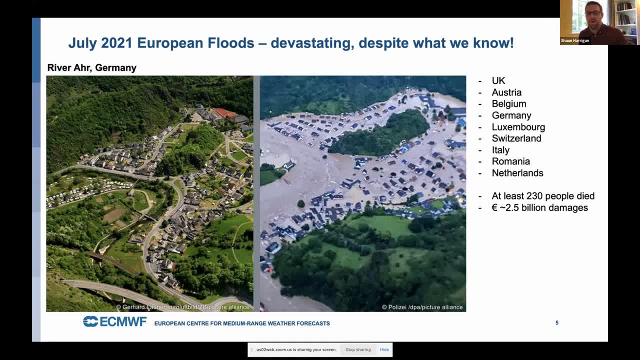 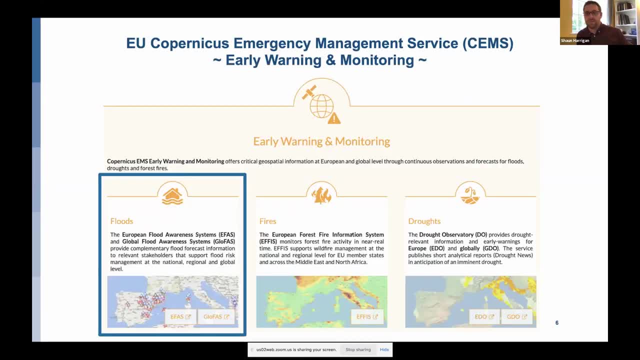 summer. so that caught contributed to probably the in a way surprise. but was it a surprise? is is also a question we've asked and this is where uh comes into our my own work. uh currently is. i work in a european commission uh project for the east and the west is the computational center. 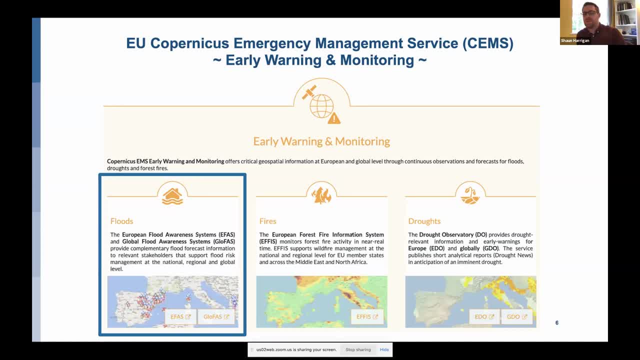 um it's for the copernicus emergency management service, so it's an early warning and monitoring service and in that we run this european flood awareness system and that some of you may or may. and if we look at just the signal from um, efas several days, so in the medium range. so you know. 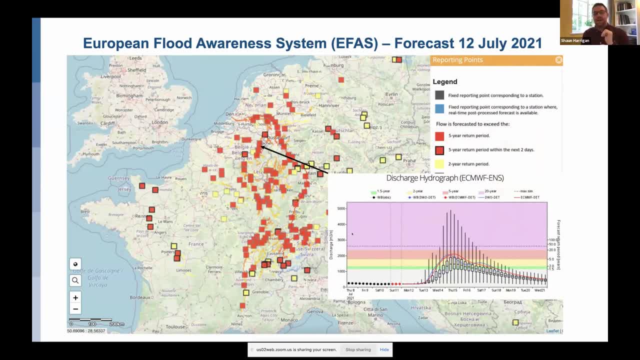 two, three, four, five days in advance, and and i i'm showing one picture here, but i've also been talking to um jury forecasters who were working in the countries and that were mostly affected and hearing their anecdotal kind of stories, and from both from a meteorological point of view and 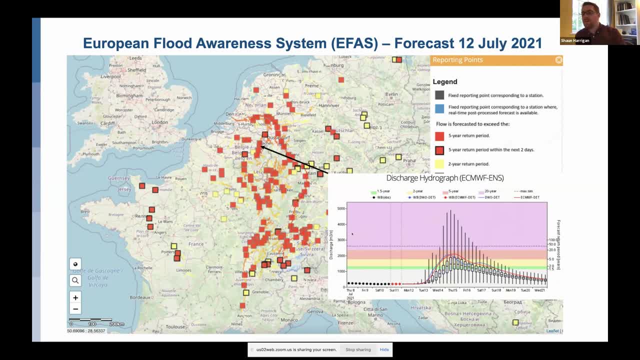 from a hydrological forecast point of view, the signal was in the system three, four, five days ahead. um. here's this one example in the river moose and belgium. um. this was uh initialized um on monday the 12th and you can see that the peak really happened on thursday the 15th, and so the signal 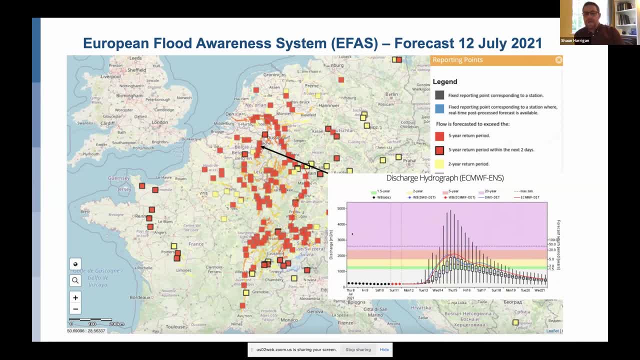 was here. it was already there several days before um, and so you can see the spatial extent of of that signal. so each um kind of red square signifies a point in the river network that the five-year flood return period has been exceeded or predicted to be exceeded. 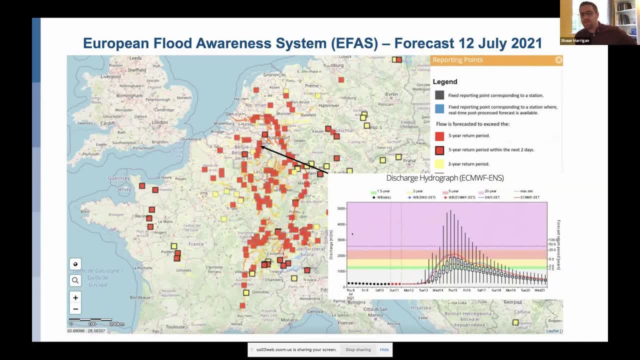 it with some probability, um, and so you can see, the special extent was already forecast in advance. we can see that there was high, uh, some members were shown very, very extreme flooding, um, and what that says to us is, you know, we're quite happy from a prediction point of view that at least the signals 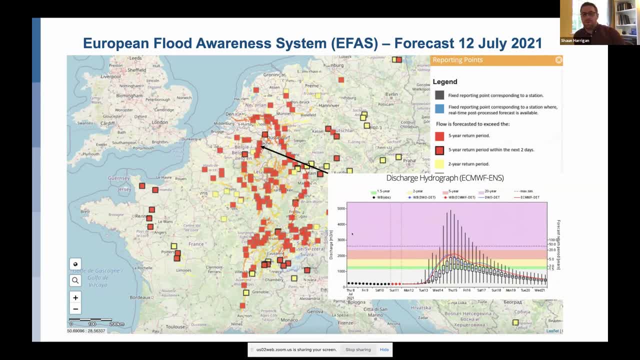 in the system, um, and from you know, our job is to provide the forecast, to provide the operational forecast every single day, twice per day, um to the the centers across europe, um, but what, what was interesting is- and it's not our role- is then the the use of that forecast for decision making on. 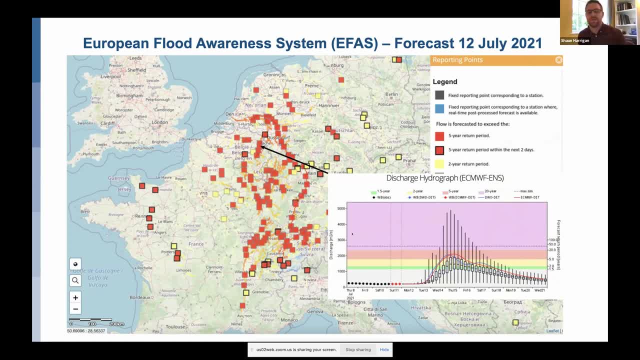 the ground and that's where, where i, i step off and that's where our job is, is not, uh, it's not included, but what is interesting is that, speaking to these people, it seemed to be that, um, a couple of key things is the fact that there was such a 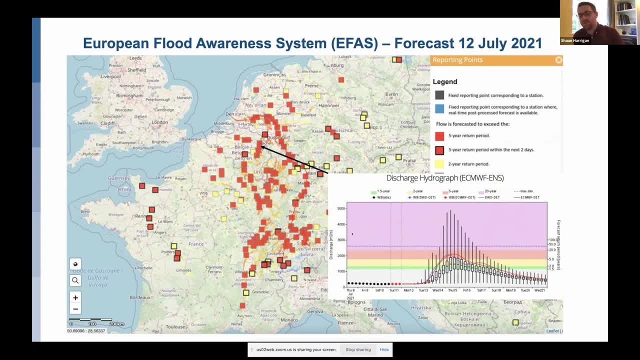 crisis of the total number of people that were affected by the flood, and there was a lot of concern about the ability of the risk. Dios knows that it's a big issue and i think next year we're hoping that there's going to be more of that risk, not only as a result of the갖bepa uh and. 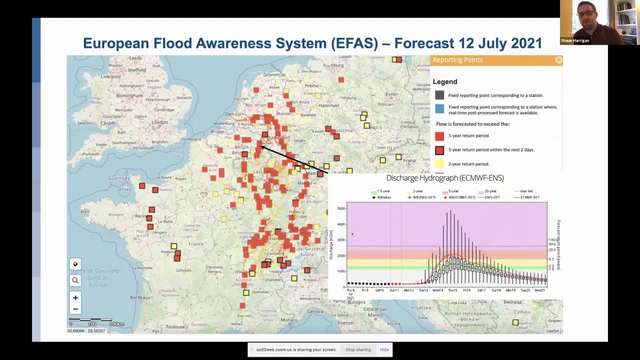 the connectivity, but also that as a result of the number of people that had to get through the flood in the area, and, uh, let's say, you know, um, it was just a pretty intense time and um, you know, you know, if you look at it from a position where, if the energy level is zero, obviously there's going, to be a lot of work. um, so if you look at the cost of it, there's going to be a lot of work. uh, so it's difficult to do. for for sure, in several countries, there was definitely things that were put in place, um, i think in july. what did? the social response was, um, i think it was the first national report of. 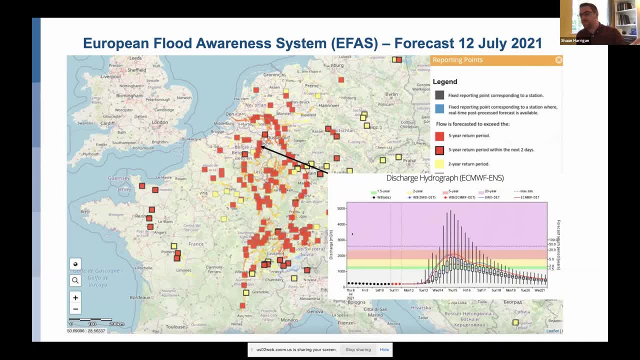 place, uh, several days ahead and as the event neared. but, as we know from the devastation, there's many, many lessons we can learn um and how science and policy and decision making come together. i think that gap is very obviously very, very wide still, and so more than from you. 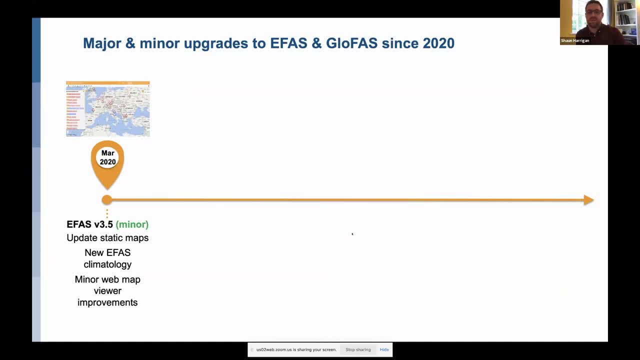 know how a system like efas or it's uh, it's uh, it's global um comparison go fast. from our point of view, then, in terms of our- my role and the role of eastern wf, you know what actually happens on a day-to-day or a month-to-month basis to keep these systems operational and working, and so i'll just 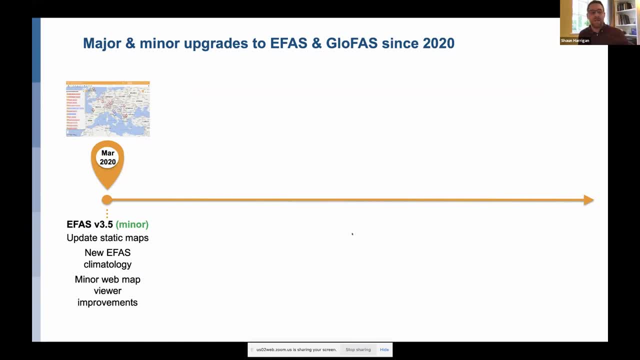 give a little bit of timeline to the last year, what we've been working on and just to show, just to give you a flavor of some of the things, so you know these systems are have been operational for quite some time now. over the last year we've done a lot of work, updating static maps to improve. 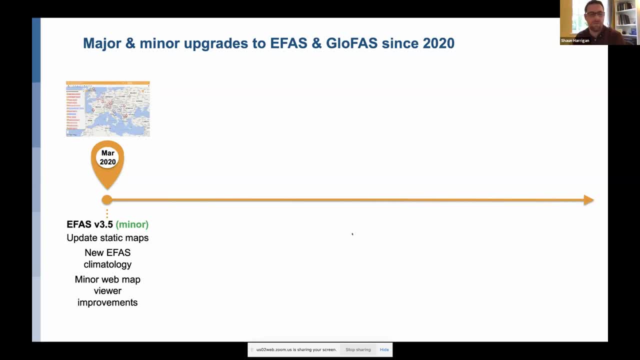 the underlying soil and underlying kind of rainfall maps, everything we've in the european model. it's been through a major calibration and so it went from a 24-hour daily time step to six hour time step across the european domain and if you see the map here on the 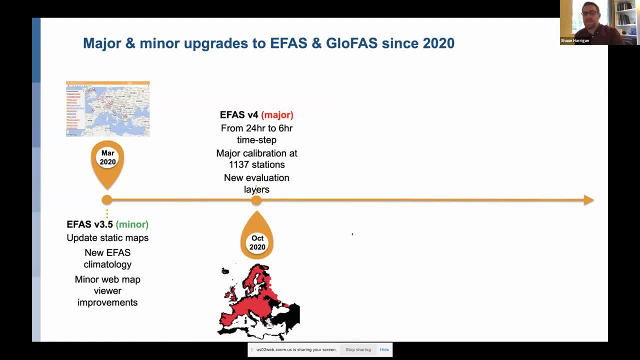 bottom um, the red catchments or area highlights um every everywhere, that the model was actually calibrated with observations, and i think that's quite impressive. it's the first time, i believe, we've had such european-wide coverage of observation um, and so that is about four million. 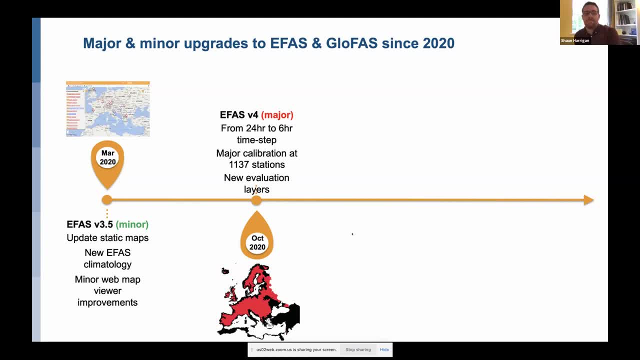 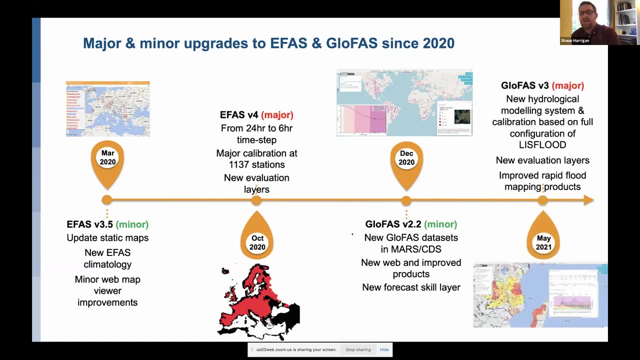 kilometers squares of an area. it was calibrated um, and so that's been operation since october. we look at our global counterpart. we've improved the web. we now have all the data from the simulations and the forecasts are all open and open access and new skill products and as well as 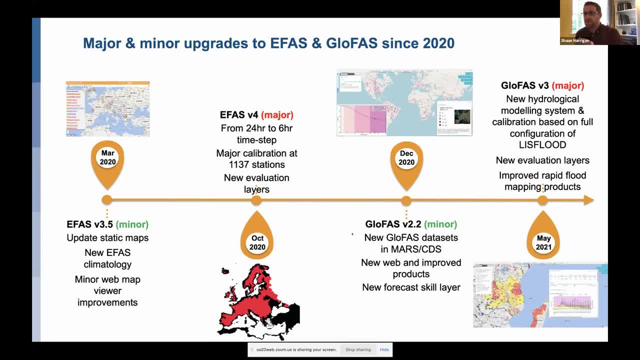 impact maps. so rapid impact mapping, so when a flood occurs, we can also get a first estimate of the damage, and so that's just give you an idea of the type of things we've been working on over a a year. it's been quite a busy year, as we know- that lead to a system that's able to predict these. 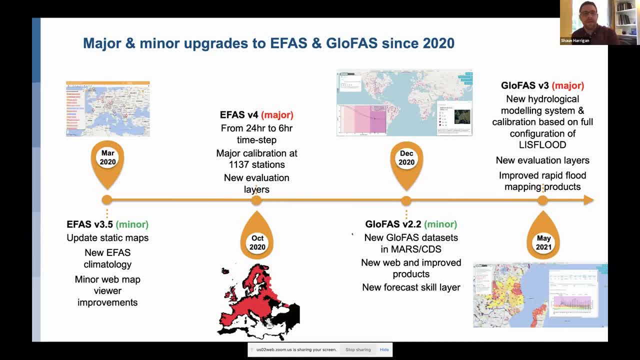 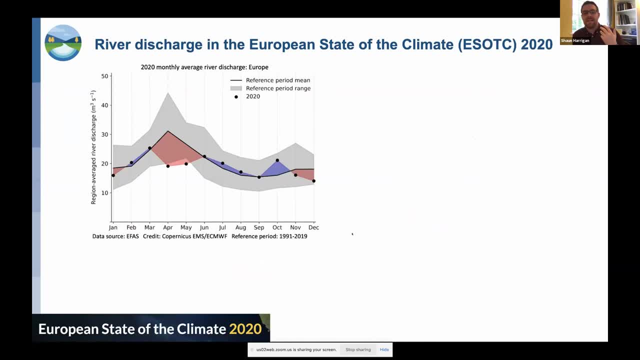 flood events several days in advance. so quite a lot of work going on underneath and i think what, what? that when we get to the point of having these large-scale systems, um, we see we can do other things like. i think what's been missing at a european scale has been the understanding of 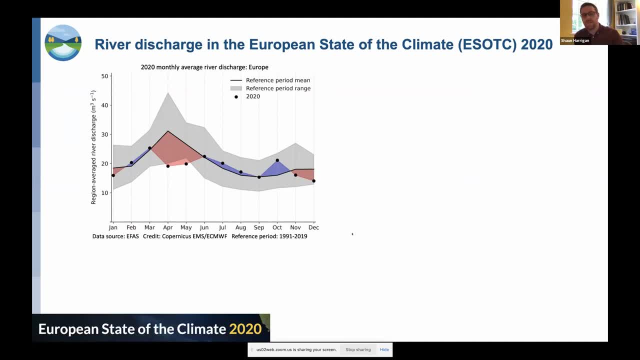 how hydrology is changing. so, yes, we have some networks and observations, and observations are are the most important thing. they're not a replacement, and assimilation cannot replace observations, but what observations can't do is give us a complete spatial temporal picture, and so we've been able to contribute to the european state of the climate 2020 report. 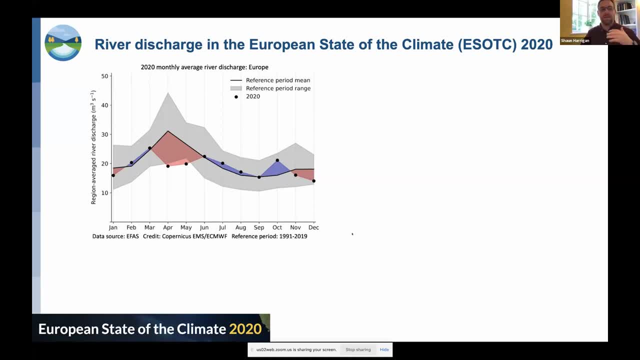 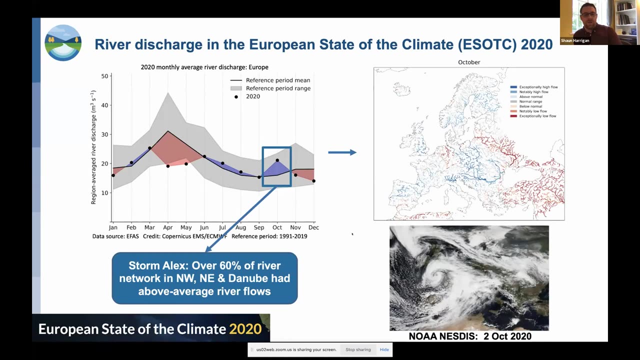 that's led by the european commission, and so we can get a river discharge, um, we can look at how river discharge has changed across europe over the last year- so in near real time essentially- and we can see different patterns of um. you know, high and low vents, and so this is just one illustration. in october, we can see the overstorm alex. we. 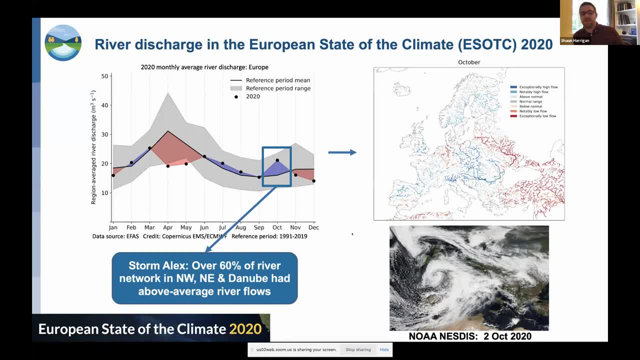 can actually get some interesting statistics. so we know that over 60 percent of the river network in northwest- uh, northeast- europe in the danube had above average river flows. you can see from the graphs to the right, and this is the type of thing that i don't think. 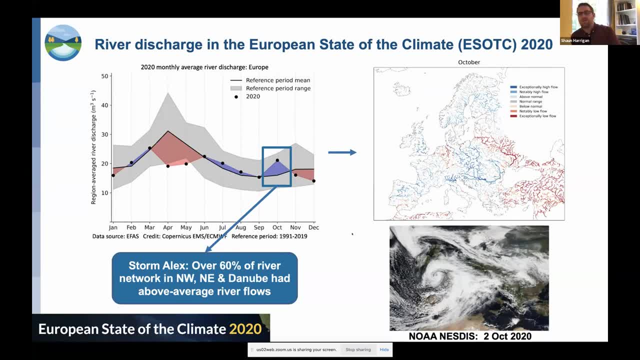 has been possible before. so i think it's quite and not a really interesting thing to be able to do to understand the spatial patterns of changes in hydrology. um, again, i do always caveat that these simulations and they have to be used within the context of what the observations say, but at least, 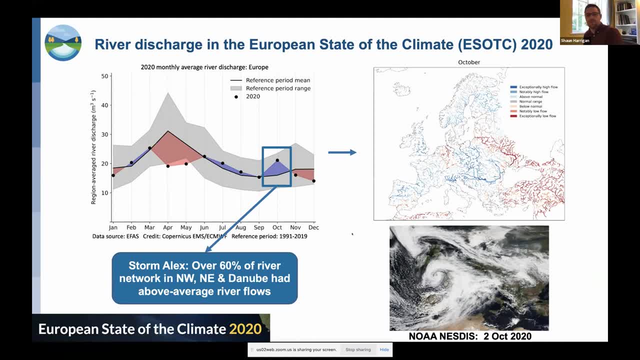 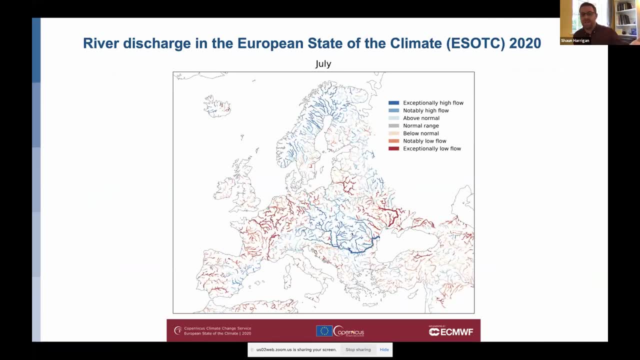 we have. it's a piece of information. I think it's it's interesting, we can use, and so we can then create things like the evolution throughout the year. we can look at what areas were exceptionally high, exceptionally low. we know that floods and droids aren't completely separate and understanding. 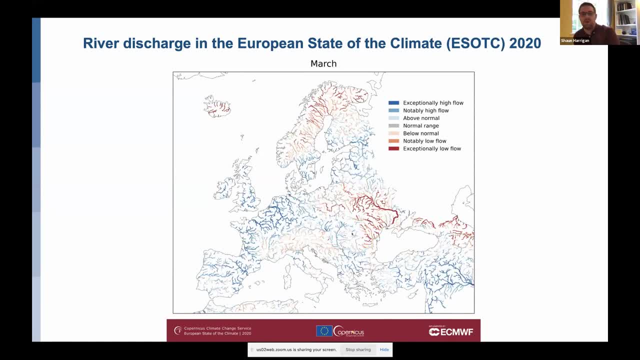 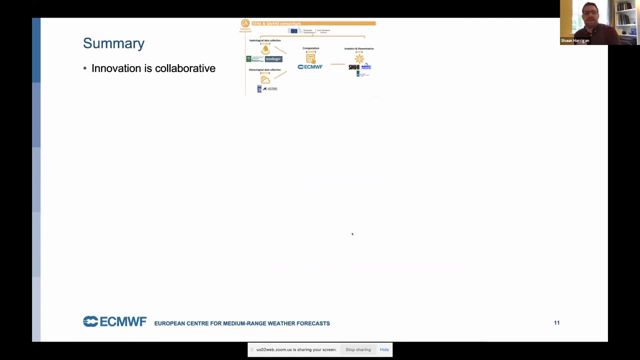 that dynamic and how it moves across the continent, I think opens up a lot of scientific questions and possibilities. so all that data is freely available and and um, completely open for innovation, I should say. and so, just to summarize, um and just you know, reflecting back in my career and reflecting 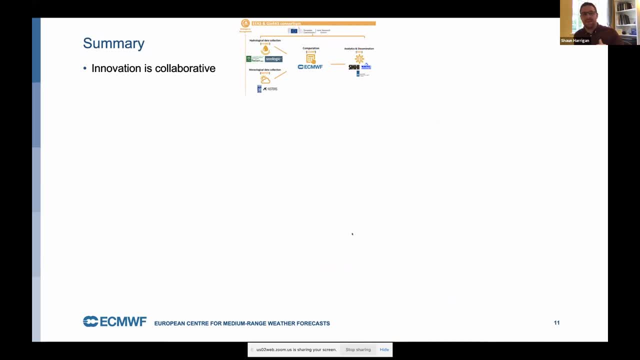 back in the work that I've done now and what, what important things, is the thing I think we've learned? as you know, innovation in my perspective is collaborative. if I look at the, the data and the systems we're running, it's it's not an individual person. it's not an individual. 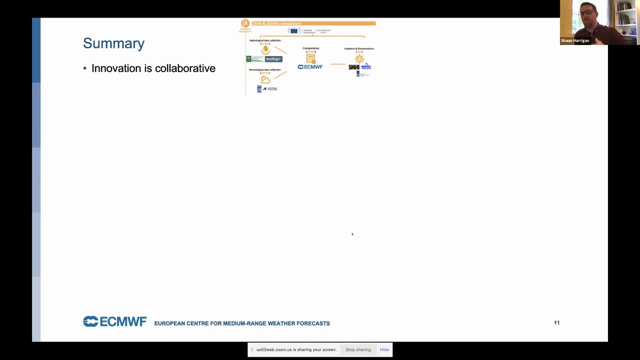 thank you, the company you know and the efas model. we have all the partner organizations across europe that give data. we have a hydrological data collection center. we have a meteorological data collection center. we have the computational and the dissemination of the forecasts, with many organizations working together to produce that. um also, i would say, innovation happens by starting. 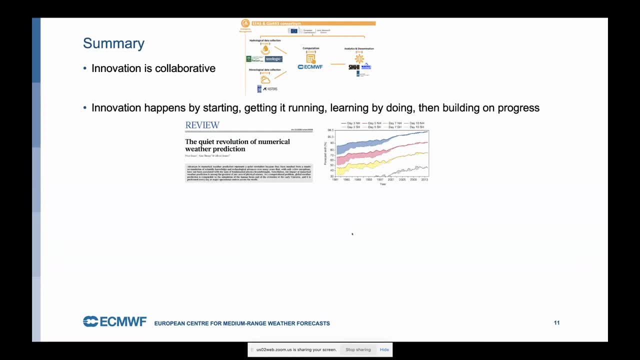 getting it running, learning by doing and building in progress. so of course, you can have these one-off fantastic ideas, and that's brilliant if you can, you know, achieve that. but i i use the, the example of weather forecasting, um, and this famous paper, the quiet revolution of numerical weather. 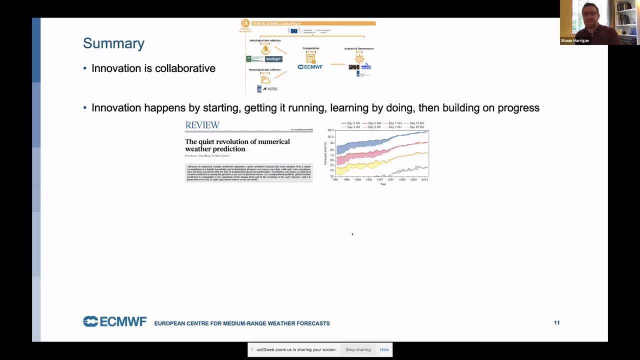 prediction. um, essentially we gain one day skill every 10 years of research development, and that might seem like very little progress. but if you look at this from the 70s, you know we can predict three, four days ahead better than we could you know 20, 30, 40 years ago. and so that is the same. 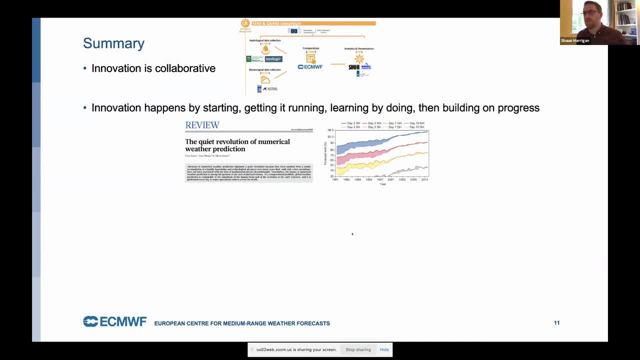 kind of um the where we are from the hydrological forecasting point of view. if we can gain one, two days skill over the next five, ten years of development and research, then that's going to help decision makers and just provide, you know, a more robust, um kind of uh set of tools. 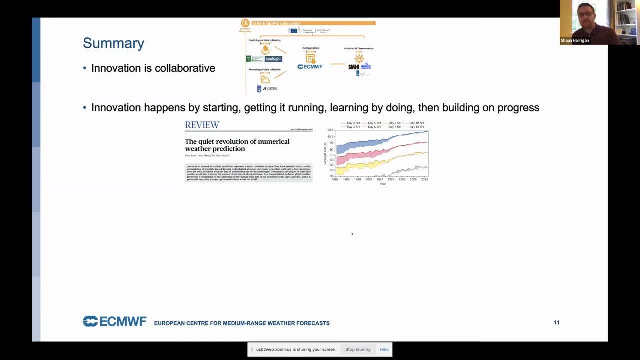 for decision makers, um, in terms of floating, as we've seen from the evidence, both observations and future, uh, this is something we're going to have to really deal with, uh, going forward, and so, finally, then, i think it's going to take a community to prepare for the. 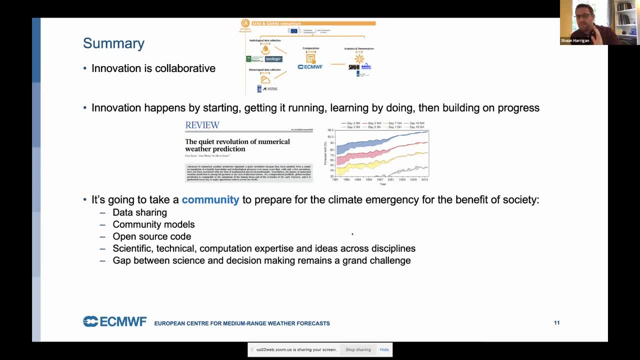 emergency for the benefit society. uh, we, we needed. we know data sharing is a huge issue in hydrology, but it's something we're getting there with slowly. surely? we know models are being developed at different places, but again, i think the more people and the more expertise we have, and expanding these. 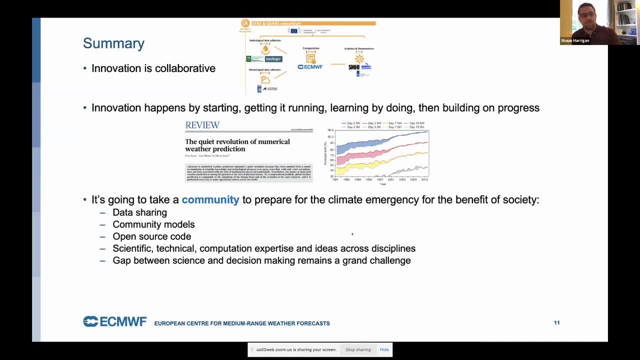 models, not just hydrology but also into the earth system, is going to be important. we've seen open source code and the benefit of that, rather than closed systems, and really it's about bringing the scientific, technical, computational activities across disciplines, and that's something that i don't think we as hydrologists can solve by ourselves. we're going to have to contribute to. 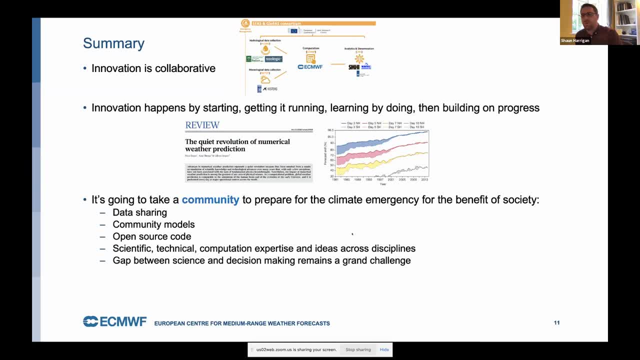 other disciplines and being at east and the bath has really taught me um. working with climate scientists and and meteorologists has been, you know, hugely um uh fruitful and uh valuable and i i think, what we've seen from the events. you know we haven't solved this problem, even though 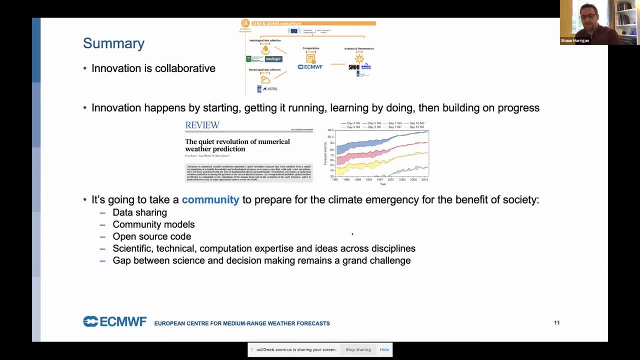 we have all these fancy systems and advanced uh forecasts from all uh, you know, from a european scale and at a local scale, we still see a gap between science and decision making, and that remains a huge challenge. so i think, um anybody here that's going to take. 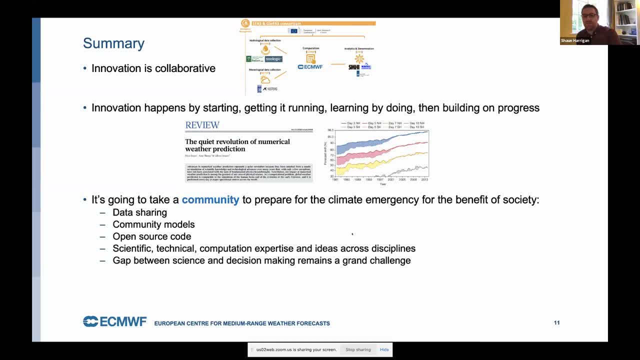 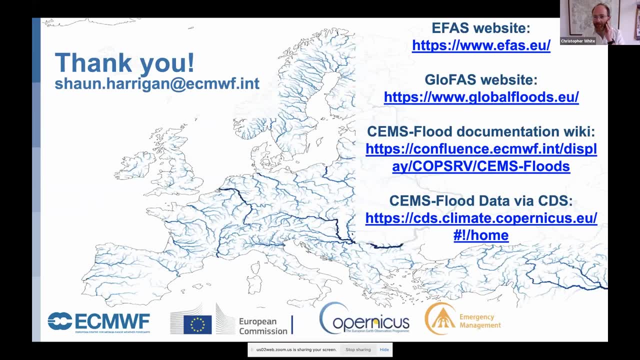 career in hydrology. i think there's plenty need for our skills. so, um, yeah, any questions happy to take, so thank you. thank you very much, sean. um uh, we're a little couple of minutes by behind schedule. um, so we'll put aside a couple of minutes here for questions for sean, please. 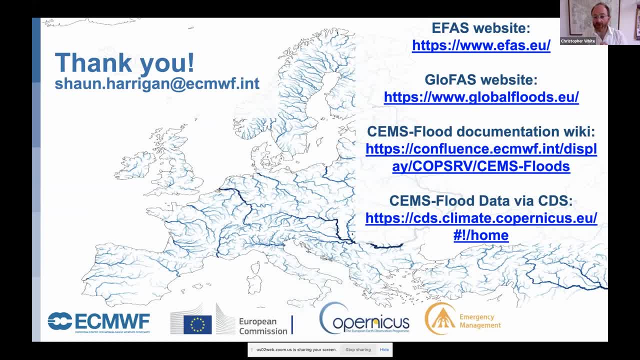 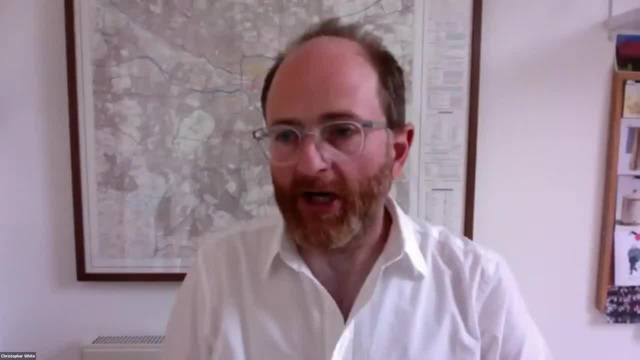 um, you can either raise your hand. we'll try. if you could stop sharing your screen, actually, that would help, please, sean. thank you, um, yeah, raise your hand and we'll try and get to you. um, otherwise, please put some questions in in the chat. so we've got a couple of minutes there, um, just while. 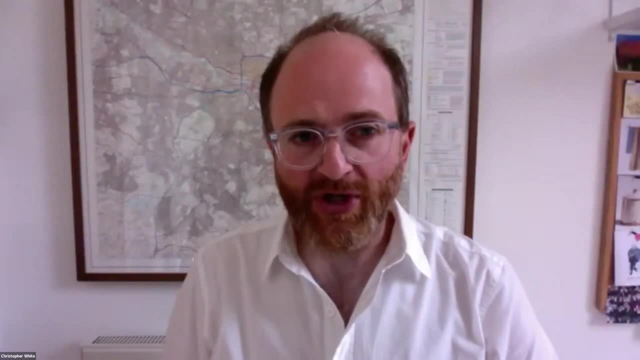 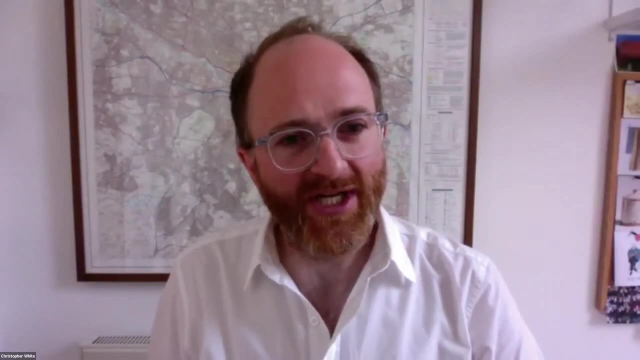 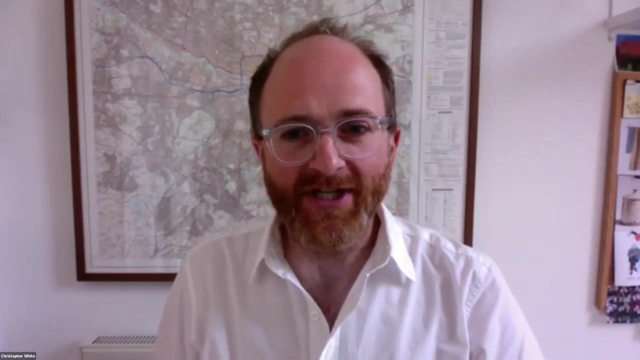 personal waiting for for that? um, you, you started off talking about your career. uh, sean, would you say that? would you say that the point you're at in your career is where you envisaged your career was going to go, or do you think it's evolved in a slightly? 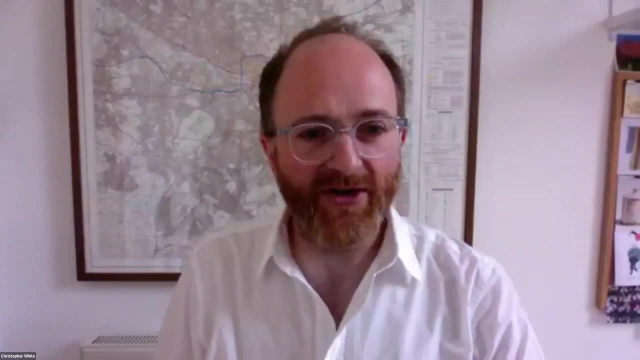 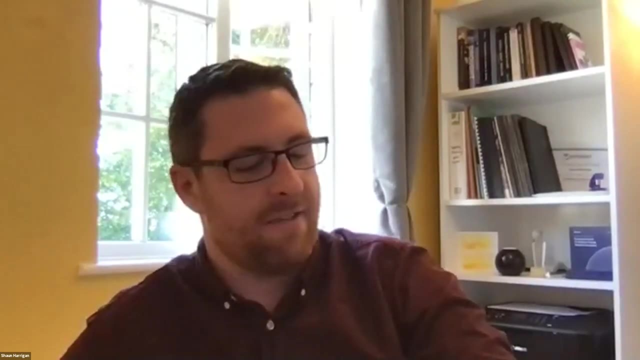 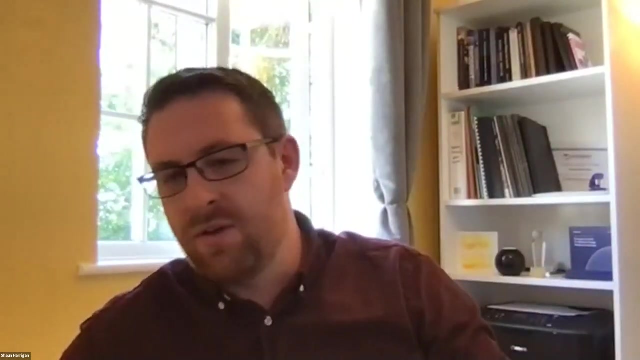 different way to. perhaps you ever thought it might have done when you, when you first set off completely i, i, maybe some people have a very clear idea what they want to do. i definitely didn't, and i think every single time has been guided by just interest. so i was interested in, you know, when a university hydrology, i didn't go to university. 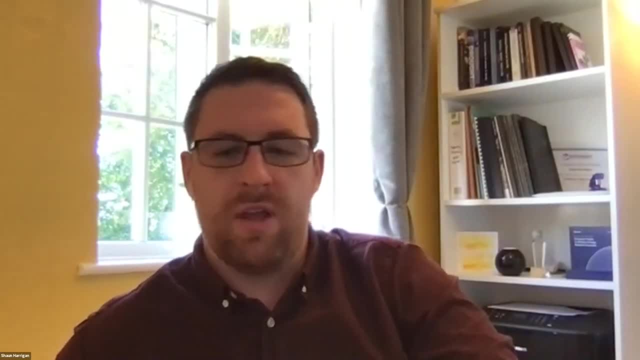 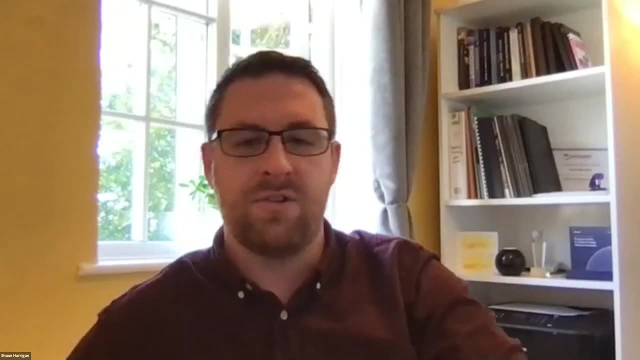 study hydrology. it just naturally happened that way. um, you know, right through to the phd, right through to even the topics you know studying at ch and then moving on. it's just interesting, hydrological forecasting. it was not something i ever even worked on, i didn't even work. 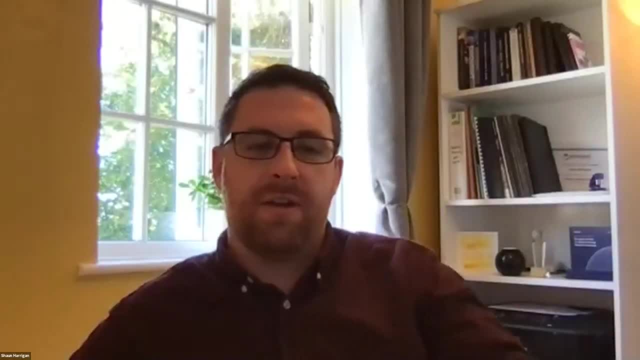 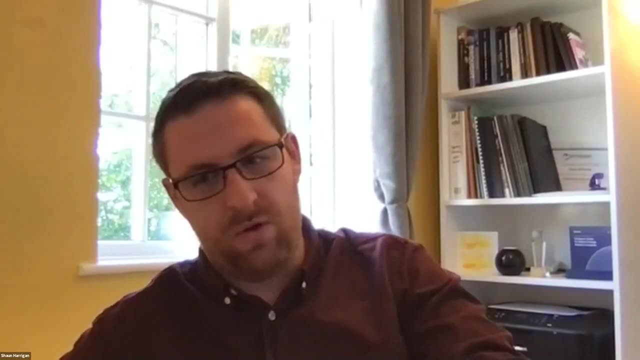 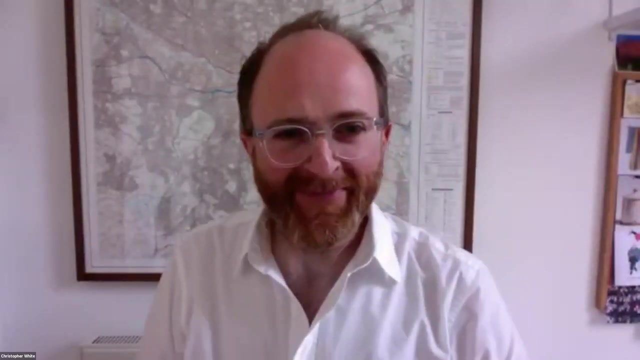 in hydrological forecasting, my phd, um, and this is not a topic i've kind of moved into, you know, being professional, uh, working in, and so i think just i've always just followed, followed the kind of path of interest and to see where it goes. there's no grand uh, no grand plan. no, yeah, and i, i 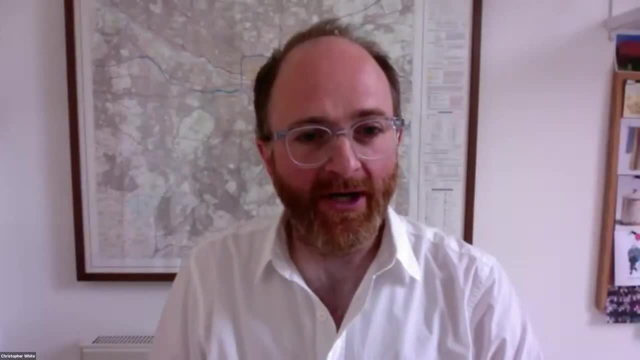 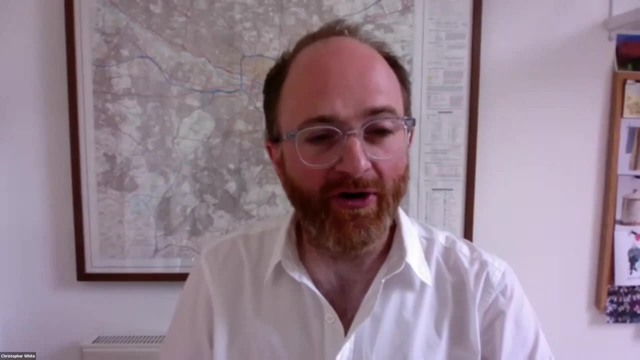 i mean, i can certainly echo those comments from from my perspective, i'm sure, probably, that a lot of us probably can, which is, um, yeah, if you're setting off in your career, whilst you might have interests and ideas where it might go, it cannot often end up in a different place, and 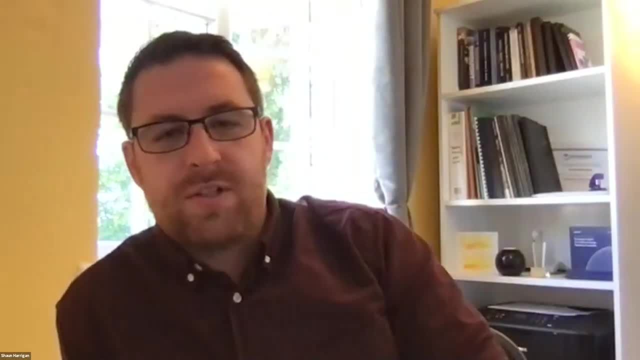 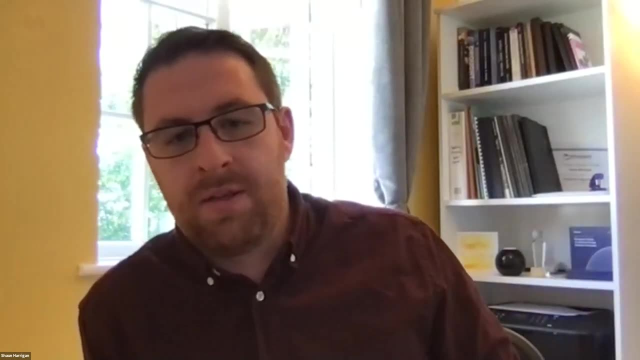 often, usually a lot better. but you know, i think the big one, chris sorry is, is that? the surprise probably is: um, i went during my phd. i just invested, i just thought i would be working academia. that's where i presumed i'd work and would be happy, and i was quite concerned moving away from academia. 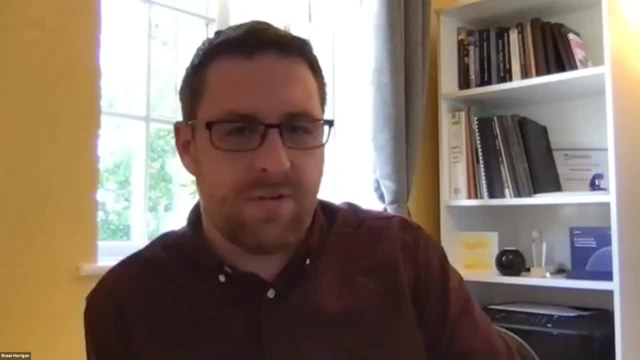 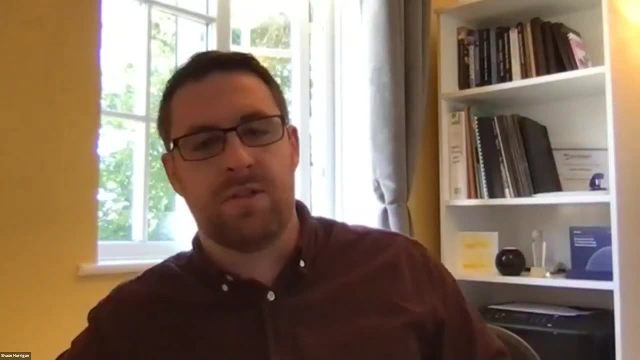 and research, and i was very grateful that i was there. um, i learned something new, which was just and well. i think that, um, like i said, you know, there's there's lots of different ways of delivering it and and there's lots of different ways of doing it. um, you know, there's lots of 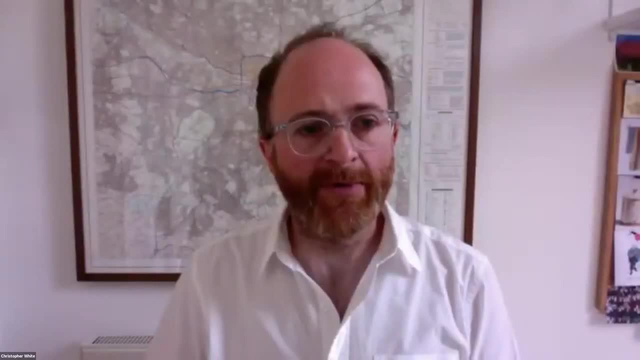 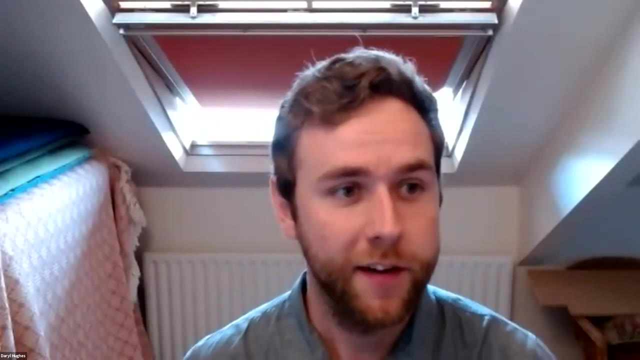 different ways of thinking about it. um, and it's interesting for me that i always wondered. i always wondered if i would be doing it for once in two years, like now. i'll be able to go back out into the field and do that, and do that again in two years, and then maybe something for all my 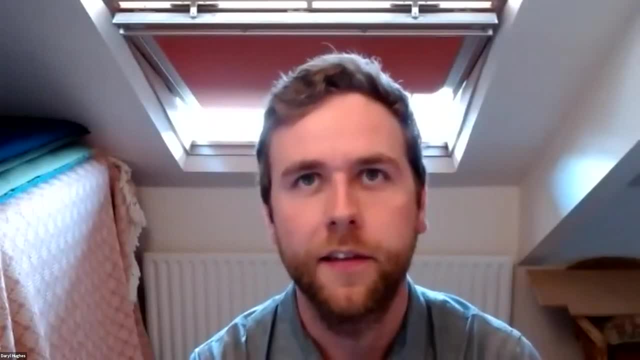 friends to do. that's interesting. that's, that's really interesting there. um, as you said, uh, a really interesting that you said. um, i was curious if you could give a little bit more insight into, uh, quid pro bono. but unless you're not a good writer and you want to put that down to a minimum, there's some. 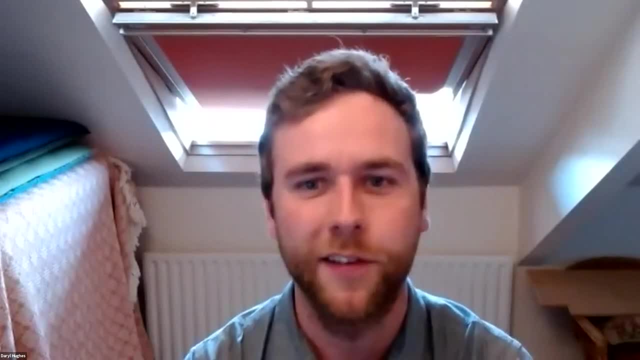 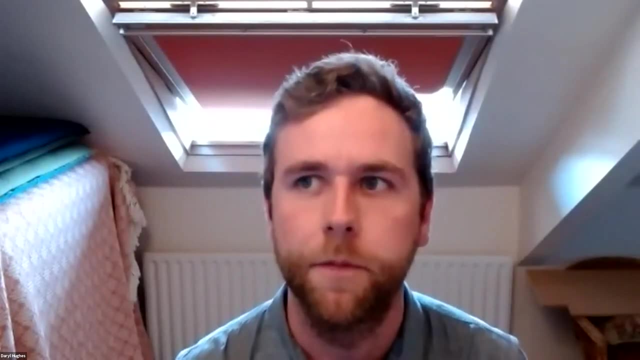 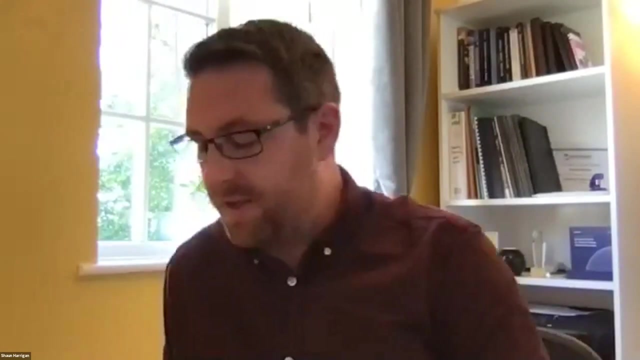 um, were you the, the forecasters encountered uh incredulity on behalf of uh decision makers and i was wondering whether you think there's a greater role for uh 3d or 4d visualization um in in combating that. yeah, i i think that's a really uh important question, to be honest, because 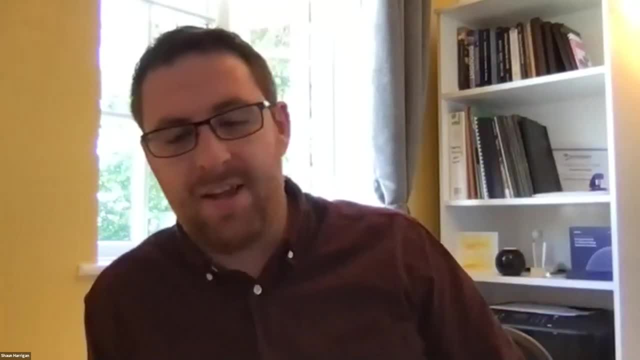 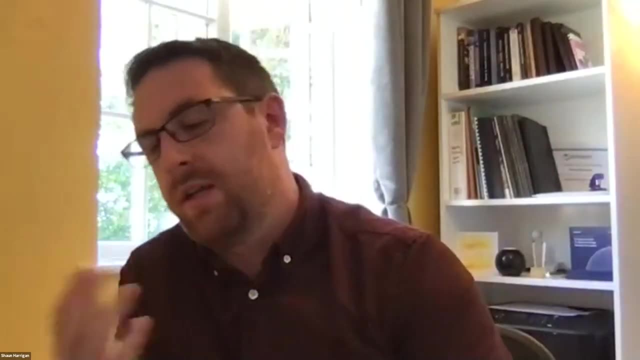 no, it was, i wasn't there. but i was speaking to a colleague in the netherlands this morning and he he said that some- he says interestingly, things have changed over the last couple of years. so he was involved with- uh, you know, essentially working with the dutch government and he said: 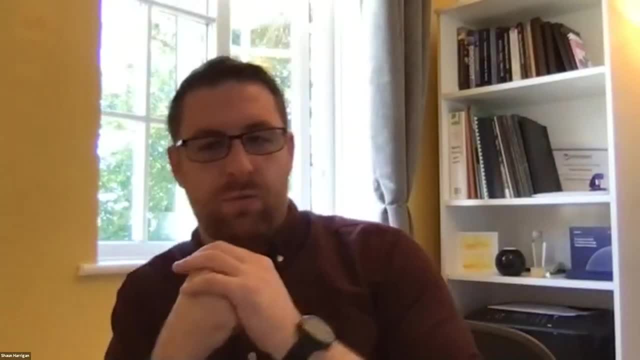 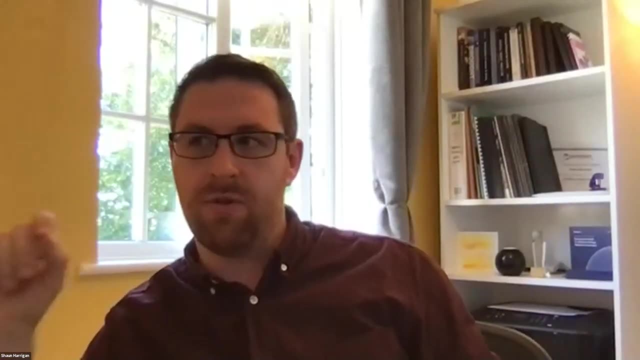 the use of, in some, the ensemble plumes, he says sometimes in the past it was always like: oh, i don't understand that. i want the number, i want that single line. we said, even though at the time, three, four days ahead, there was a small 10, 15 probability of a really significant event. 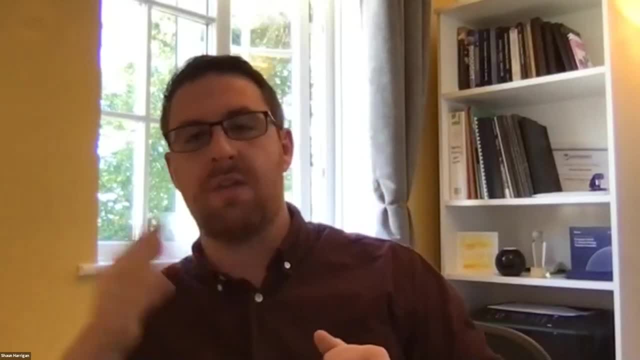 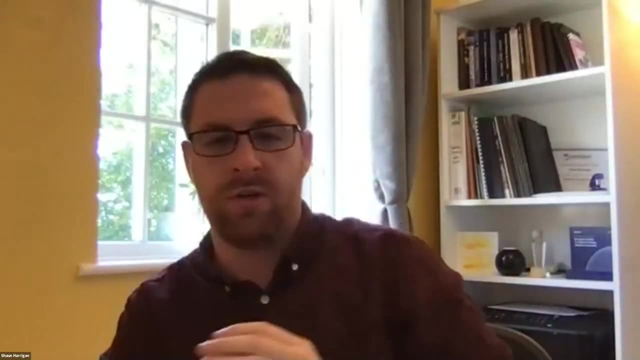 that changed. he said it didn't happen that one meeting. it took several days but as the, as the forecast developed and as the ensemble plume kind of changed and merged, you know, as it got more certain, that really set the kind of the tone of the discussions. but i think you know that's. 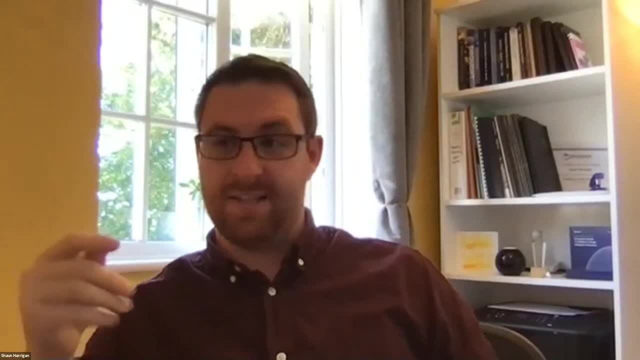 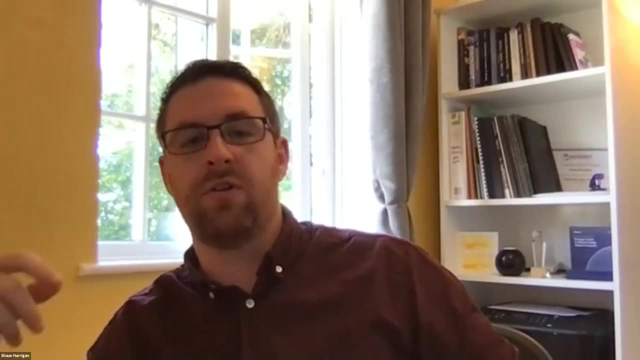 one way we do it. i think there's many. i think that, as he said, so essentially, that that was a visualization that set the discussion and so we can improve that element of how to understand the probabilities and uncertainties in our forecasts to local decision makers or to people on the ground. 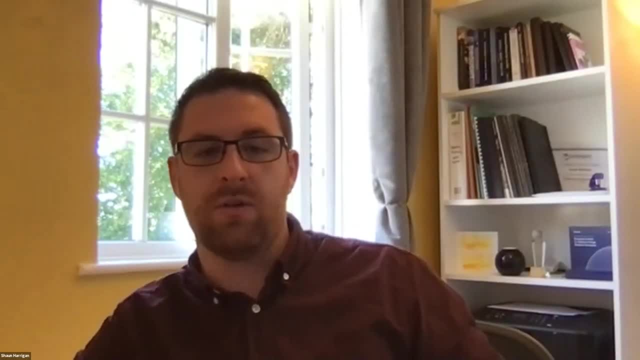 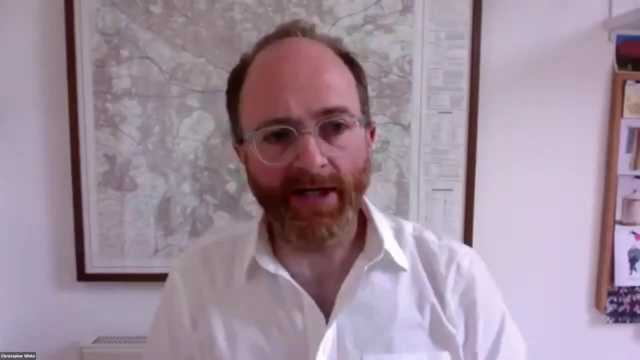 and do better at that. i think that will be one very important step to to make big inroads. so, yeah, good points, definitely. thank you uh, thanks daryl and thanks uh sean. um, just with an arm time we are running a little bit high and so i think. 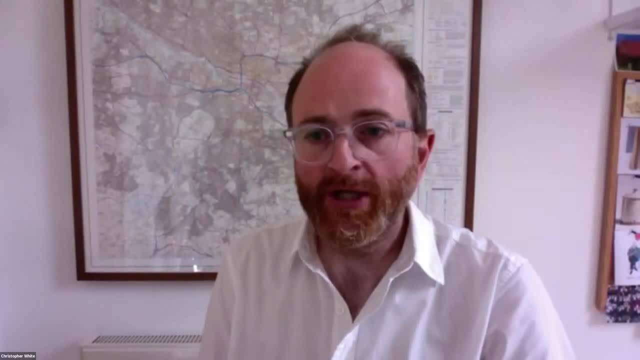 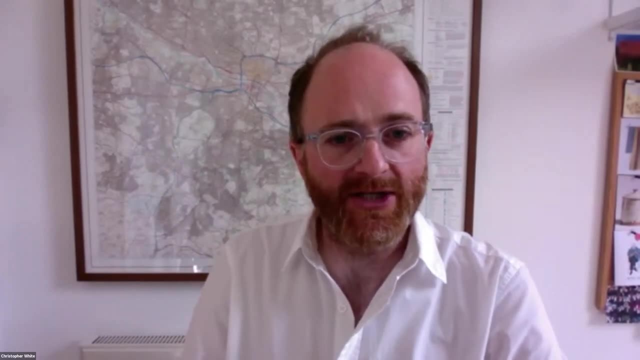 we'll. we'll call that, uh, your part to a close. but thank you very much, sean. um, there may be a couple of questions that might come sort of your way in the pound discussion at the end. but, um, i think that's that's you. thank you, um, we're gonna try again now with uh linda spate, who uh